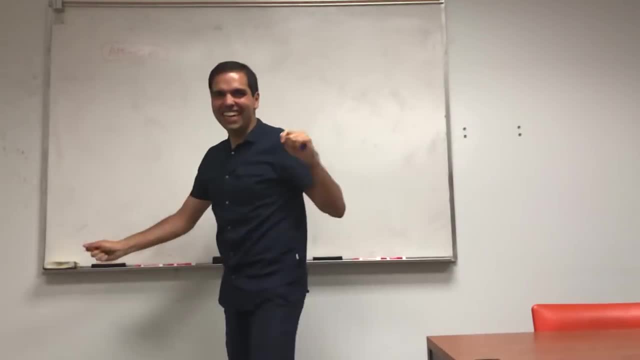 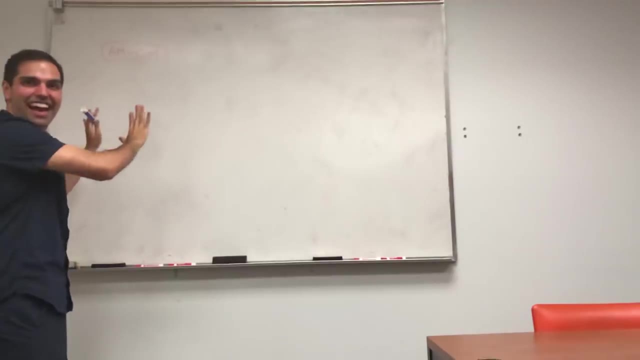 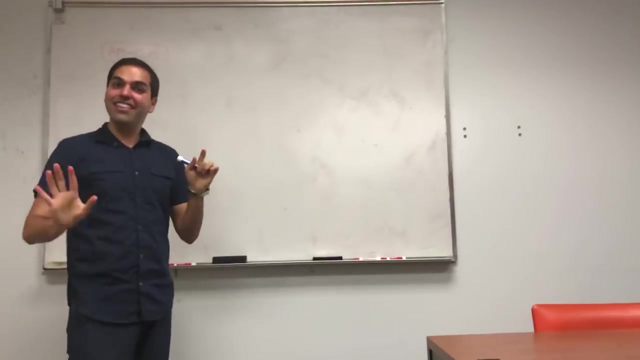 Thanks for watching and I am back. Thank you for all your patience. My multivariable class is done, I'm done with my conference and now I'm back on YouTube And, in fact, since I taught a lot of multivariable, this gave me a lot of ideas. In particular, today, let me present you a very slick 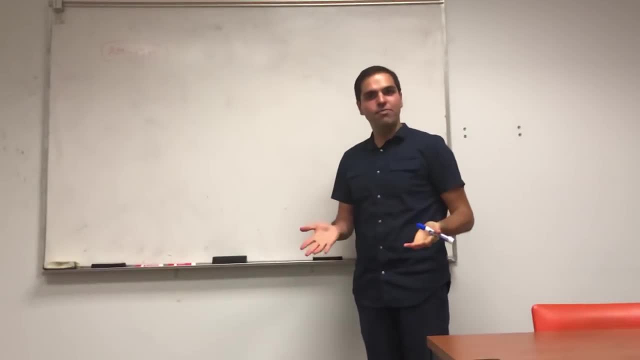 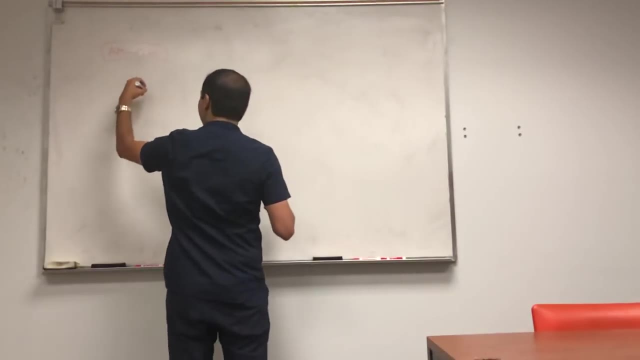 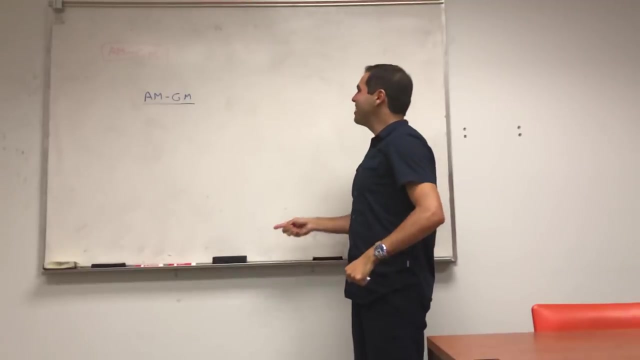 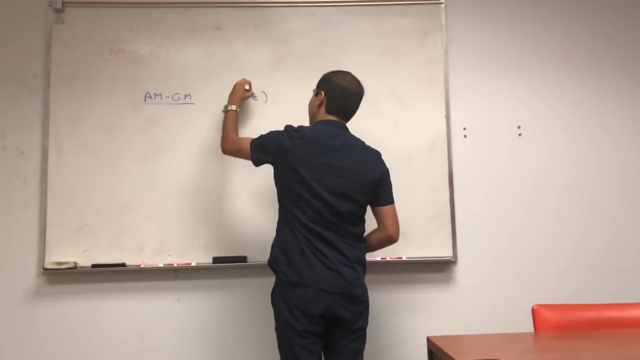 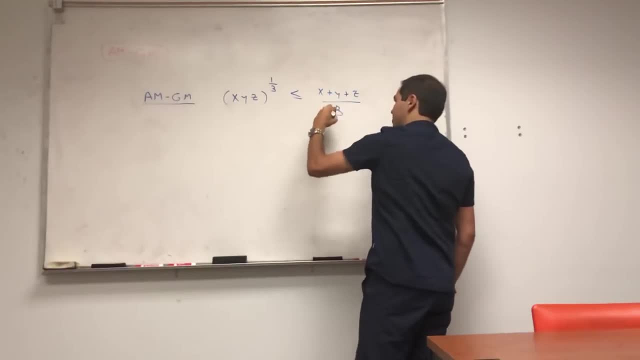 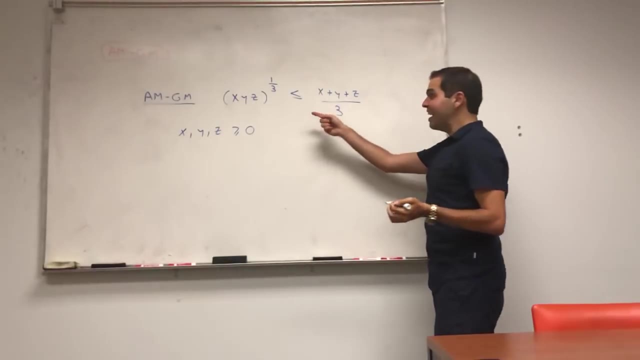 So in three dimensions it says that the cube root of xyz is always less than or equal to x plus y plus z over three, where you know x, y, z are non-negative. And this is kind of neat. It says that the geometric mean which is the cube root of the 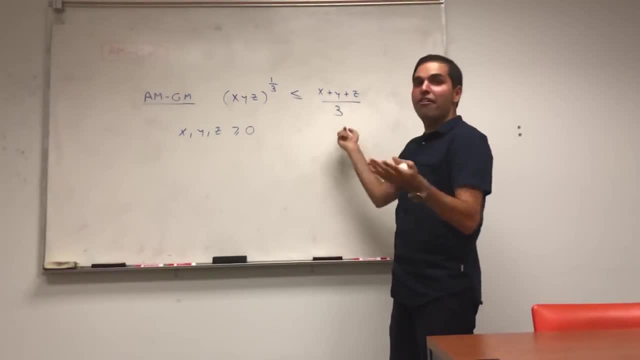 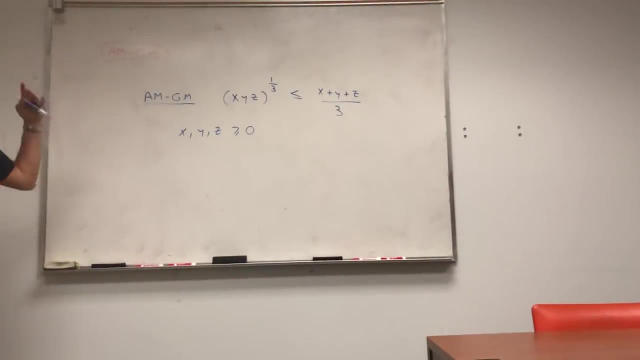 product is always less than or equal to the arithmetic mean, which is just the average, as we know, And so the way we do this. again, there's another video that uses just single variable calculus to do it. Now we want to do multivariable. So step one: 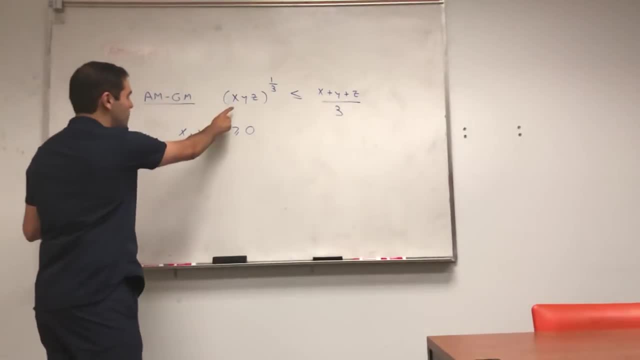 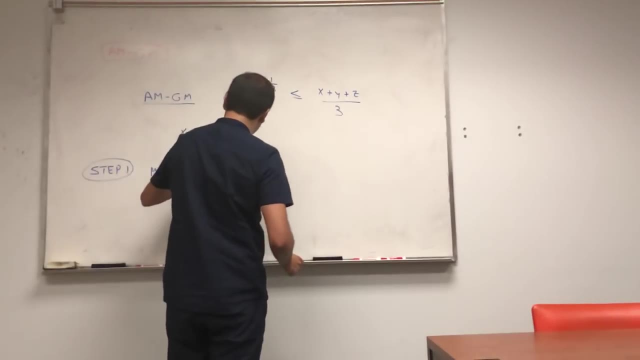 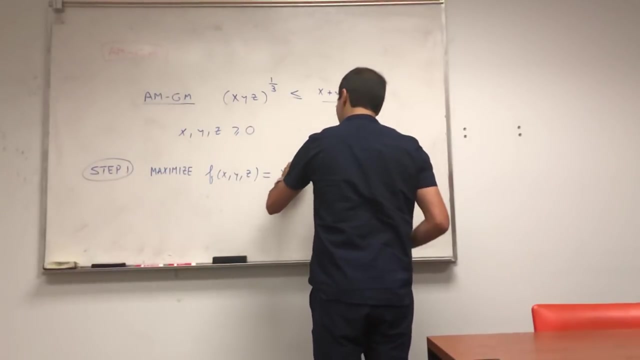 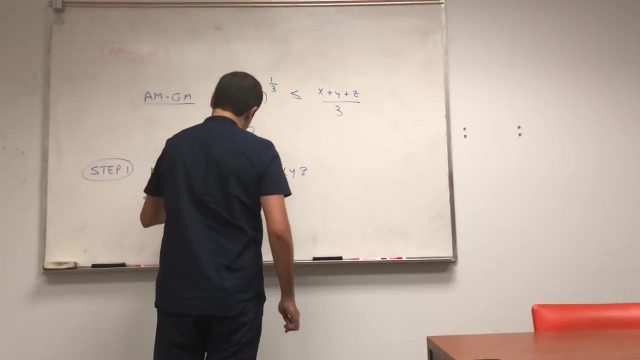 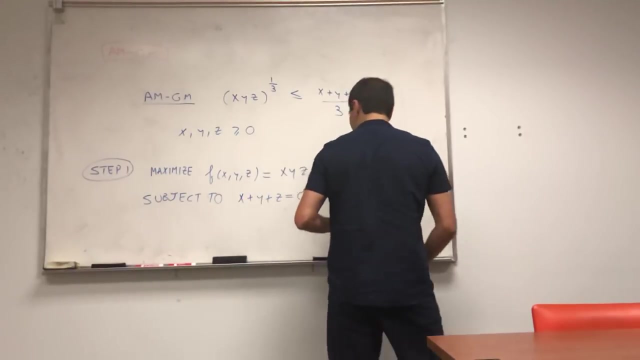 and again, it's not clear why we approach it this way, but what we want to do. we want to maximize the following function: xyz, which is just xyz. So, subject to the following constraint: we want to maximize the following constraint: two, I guess x plus y plus z equals to c, Where c is just an arbitrary constant. 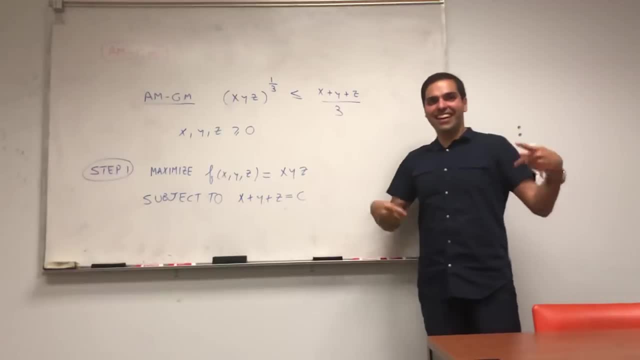 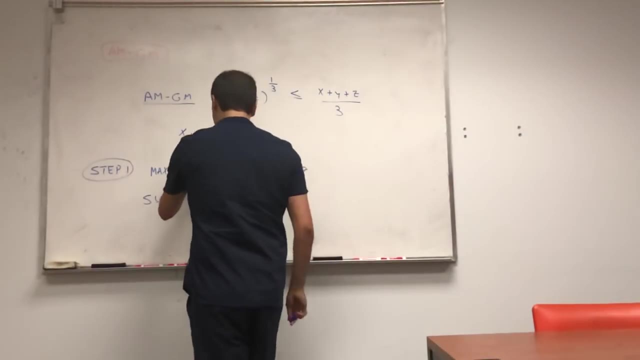 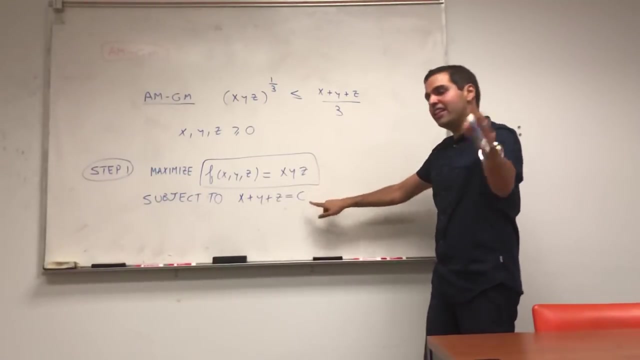 And again you might be like why do we do this? And my students at the final were also like why do we do this? But you'll see in the end what we have to do. So we want a maximizing this function subject to that constraint. so for the constraint, just put. 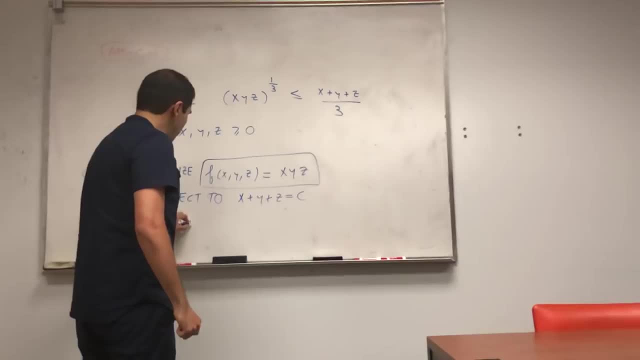 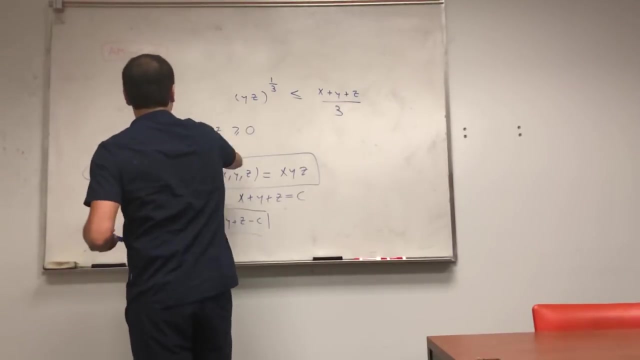 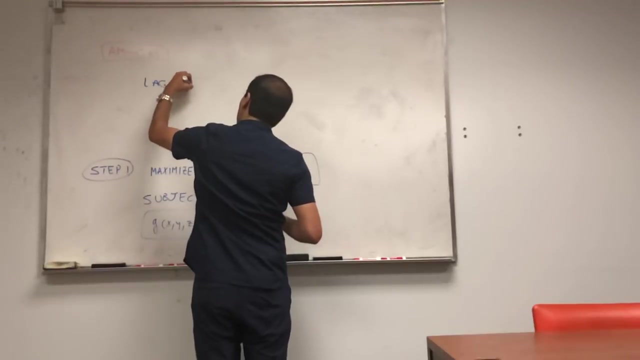 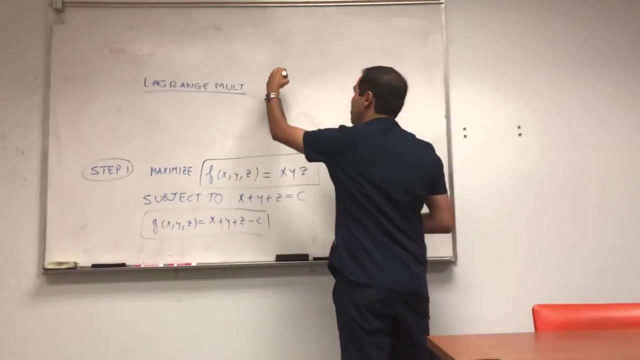 everything on the left hand side which you don't really need to do. but let's just be systematic. so this is our function F, this is a function G, and now we want to use Lagrange multipliers, which says the following all it says that you know, at a maximum or a minimum, the gradient of F equals to. 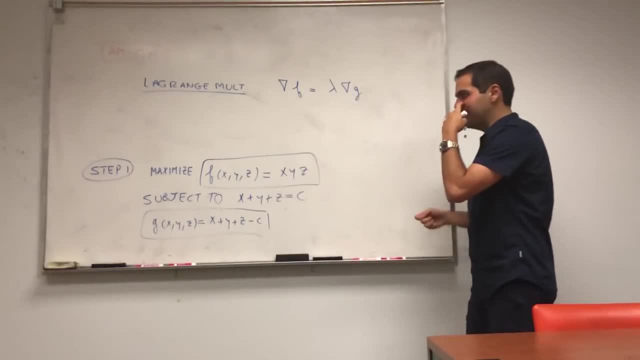 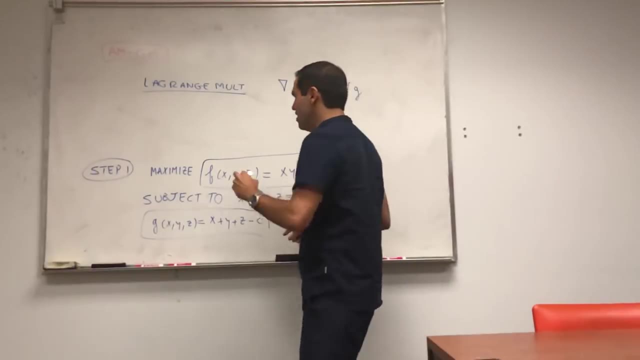 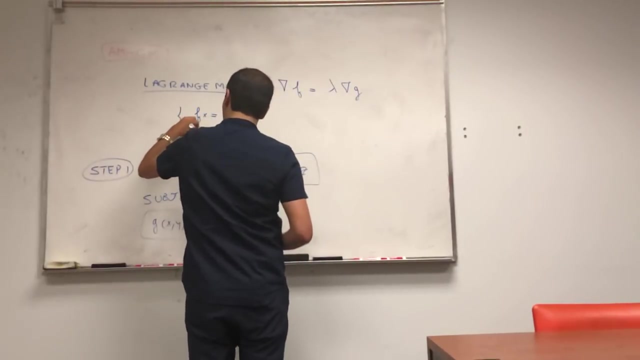 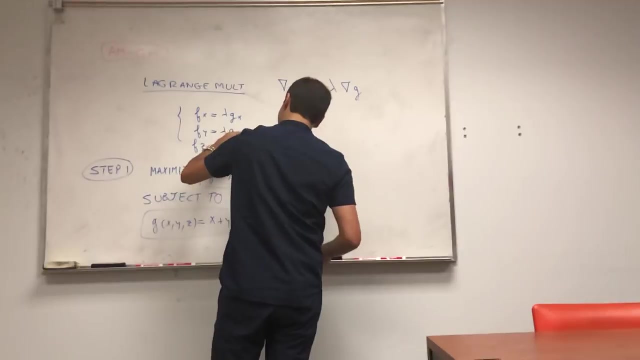 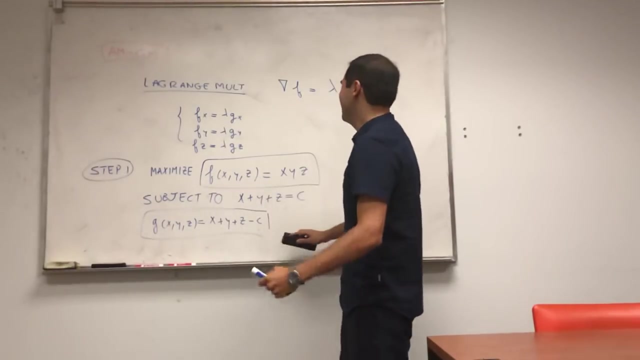 some constant lambda times. the gradient of G, so the two gradients are parallel, but this is a completely different story. so in this case, what this says is that FX is lambda GX and FY is lambda GY and FZ is lambda GZ, so it's not JZ but GZ. okay, don't you miss me. okay, well, I get. 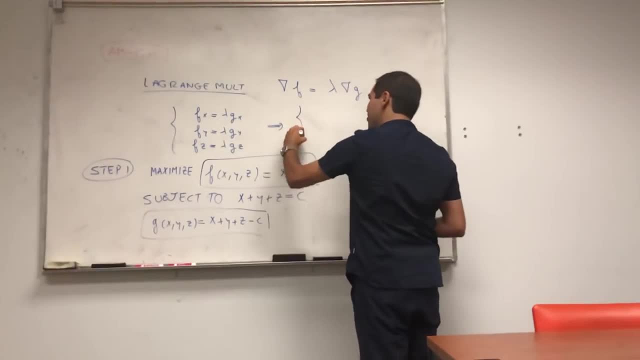 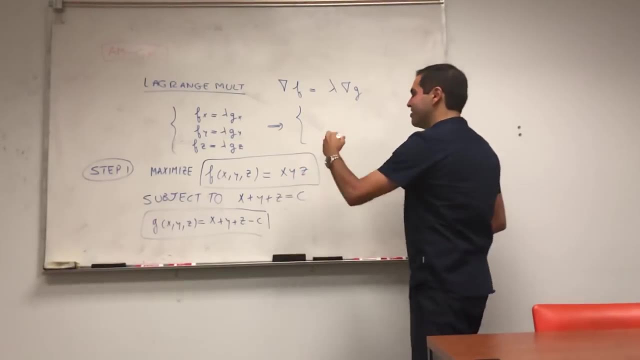 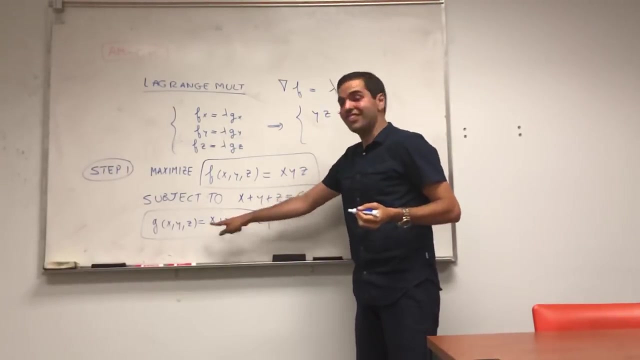 horrible equations. it turns out it gets faster. okay, well, I get horrible equations. it turns out it gets faster. okay, well, I get horrible equations. it turns out it gets faster. simplified, so the derivative of XYZ with respect to X just becomes this constant YZ. the derivative of G with respect to X, just one. so lambda times one. 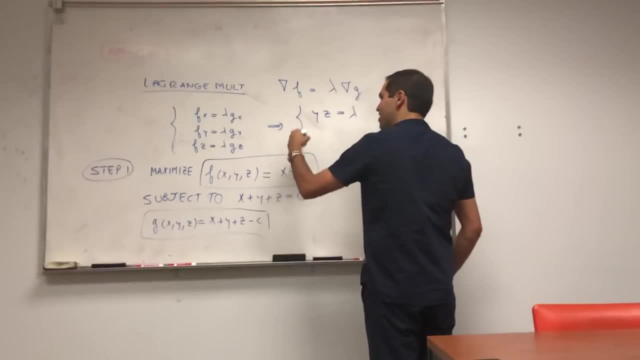 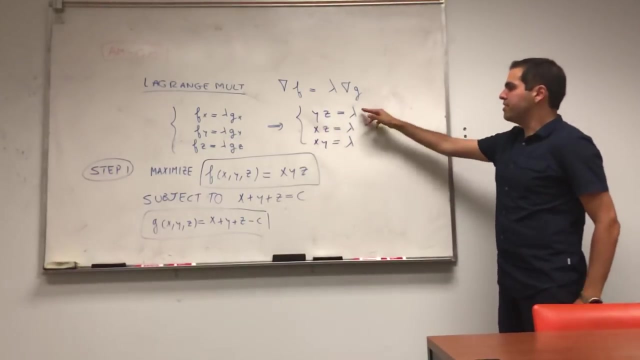 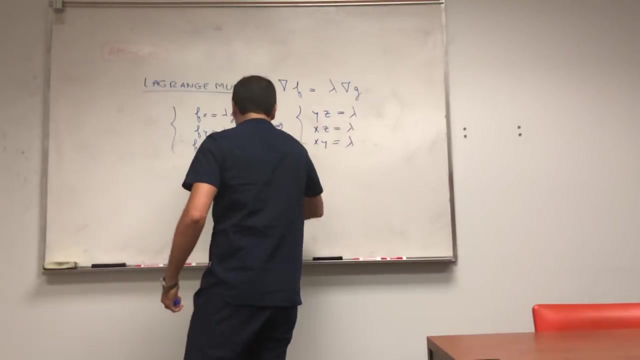 and then, similarly, the derivative of F with respect to Y is XZ, and that's lambda. and then the derivative of F with respect to Z is XY, and it also equals to lambda. so what we get is that all those three quantities are equal to lambda, so in particular, they are equal to themselves. so what we really get is: 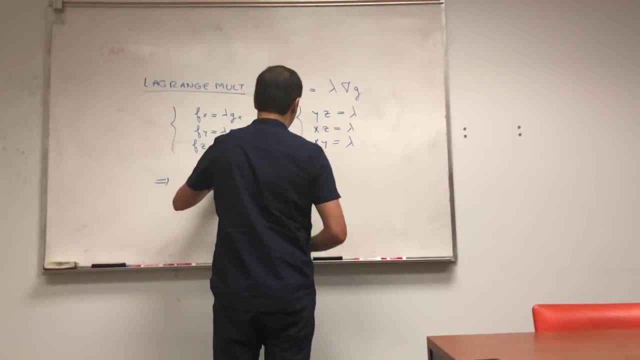 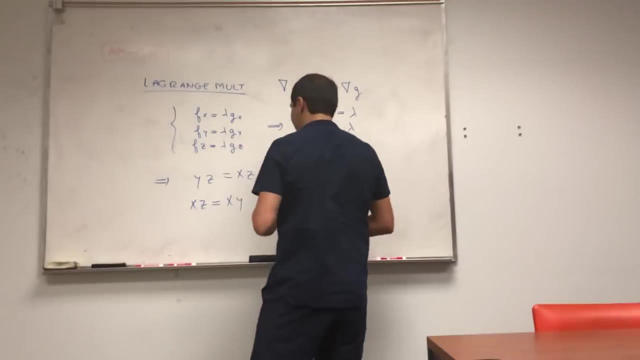 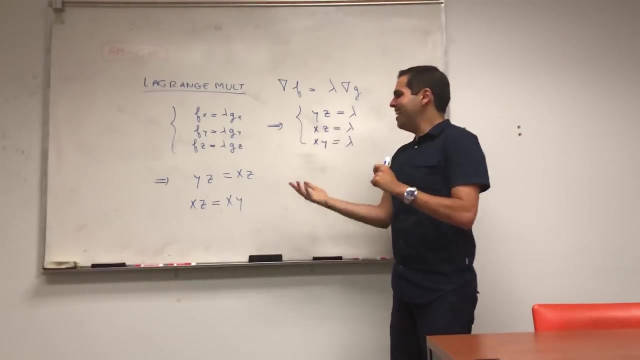 that YZ equals to XZ and, for example, XZ equals to XY. okay, now we want to cancel a, the Z's, for example, and here, and the only condition is: well, we want Z to be greater than zero, but we, it could happen that you're equal to zero. but look at. 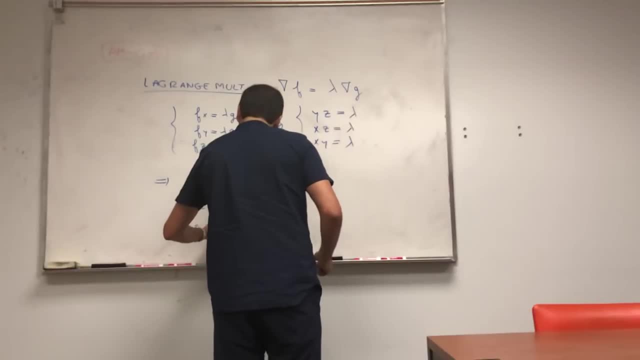 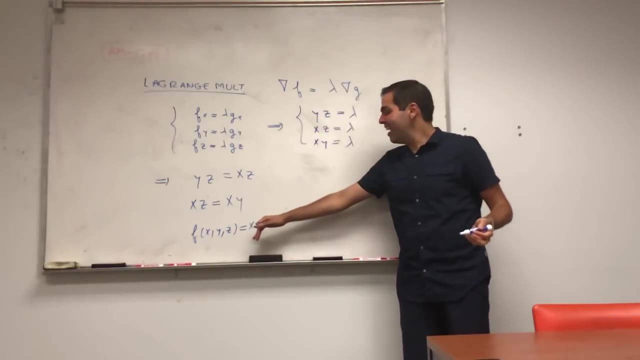 this function. remember F of XYZ, that's XYZ. well, we want to maximize this. and well, if Z is zero, then this whole thing is zero, which is not a maximum, because you could have any other positive value which will give a bigger value for F. maybe I forgot to mention that constant C is greater, or 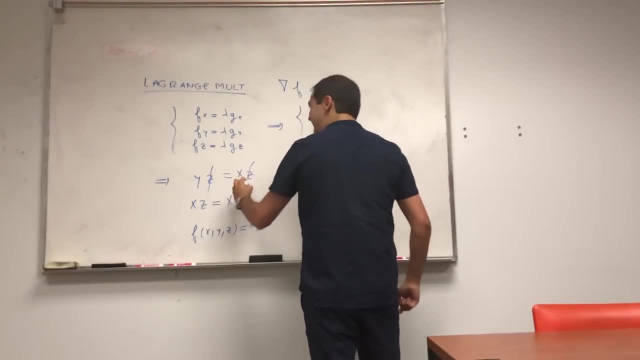 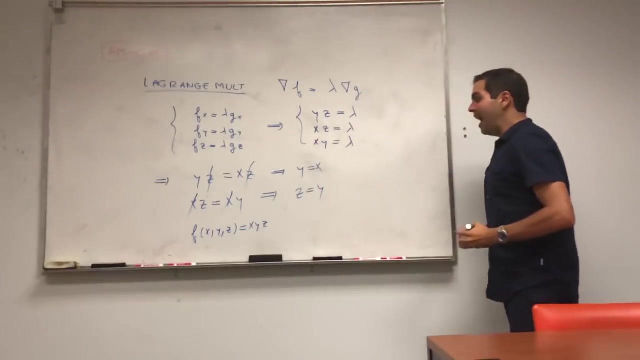 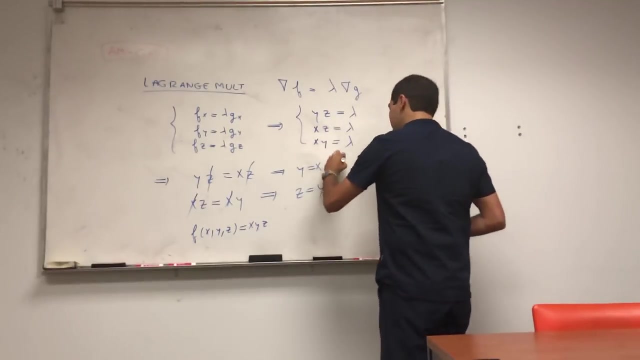 equal to zero. so we can do that, which means: now, bang bang, we can cancel that out, Y equals to X. and also similarly here, bang bang, cancel the X out and we get Z equals to Y. and lo, and behold what do we have? we have that X equals to Y and Y equals to Z, so in fact, X equals. 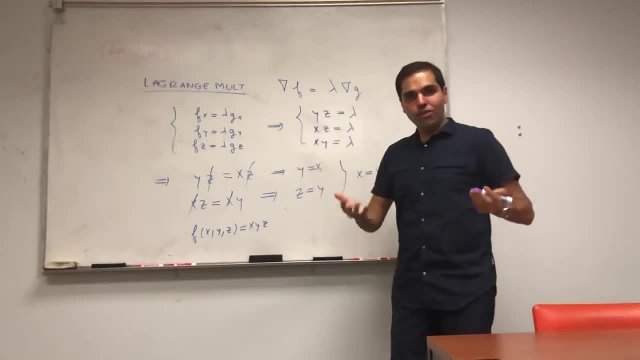 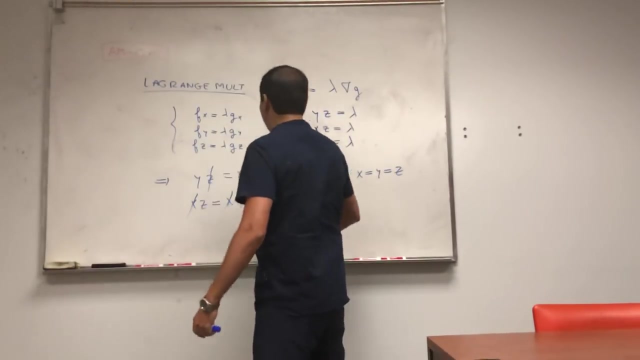 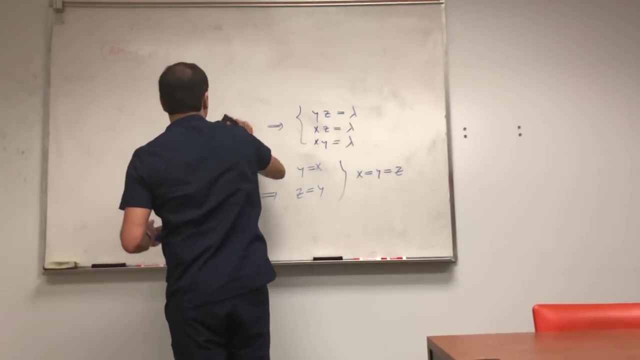 to Y equals to Z, which tells us at a maximum or a minimum. all those three quantities are equal, but the question is: what are X, Y and Z? and for this, as is usual with Lagrange multipliers, you just use the constraint, and so remember what was our constraint. 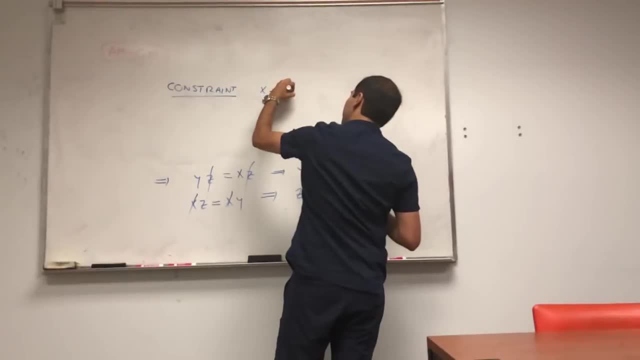 simply that X plus Y plus Z equals to C. now let's plug in: X equals to Y equals to Z. so X plus X plus X equals to C. so tres X. okay, three X equals to C and therefore X is zero over three. but remember: X equals to y, equals to Z, so Y is C over three and Z. 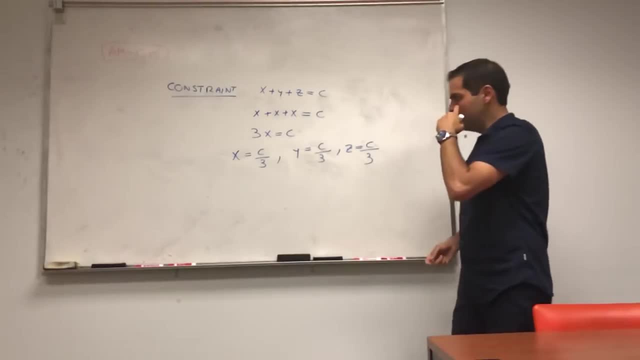 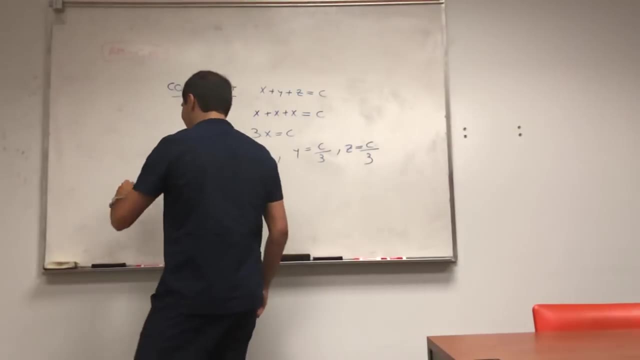 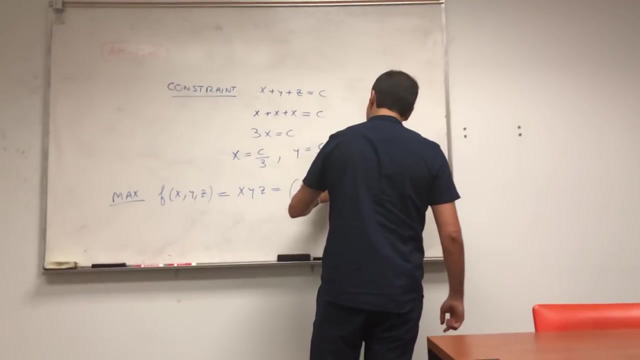 is C over three. this gives us a point where we have, you know, a maximum. but the question is: what is the maximum? well, I'll just plug it into F, so f of XY, Z is XYZ, and that's C over 3, C over 3, C over 3, and let's just leave it like C over 3. 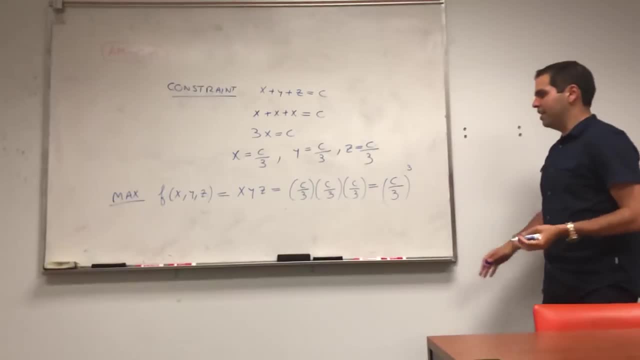 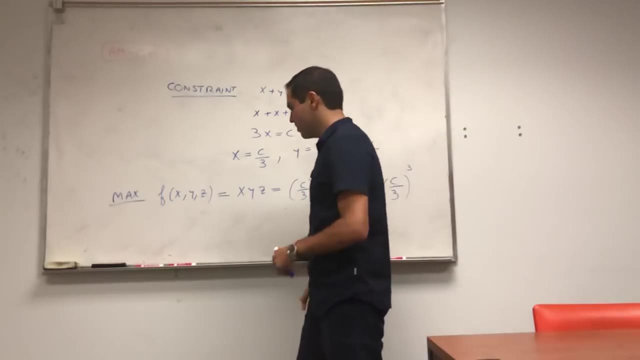 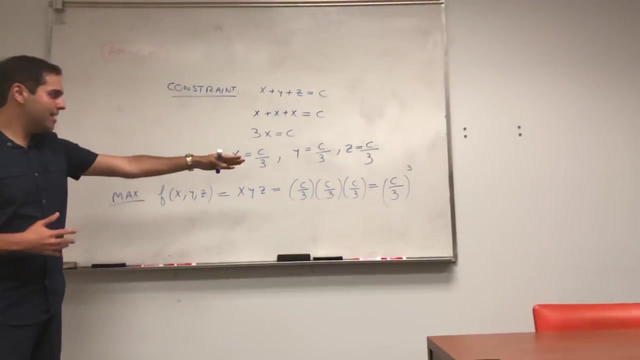 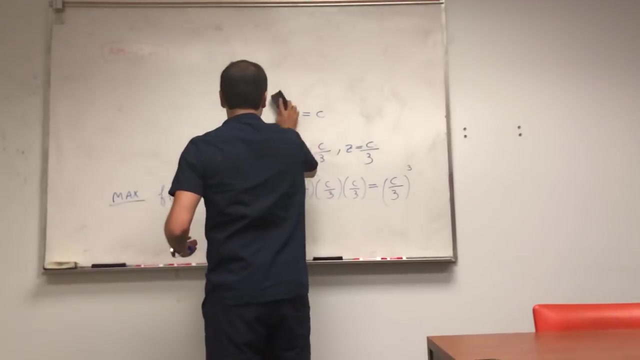 cubed. and again, this can't really be the minimum, because, if you look, the minimum is just 0 in this case. alright, so that's great. what does that tell us? it tells us that the maximum value of F is C over 3 cubed. and now, in the next step, let's. 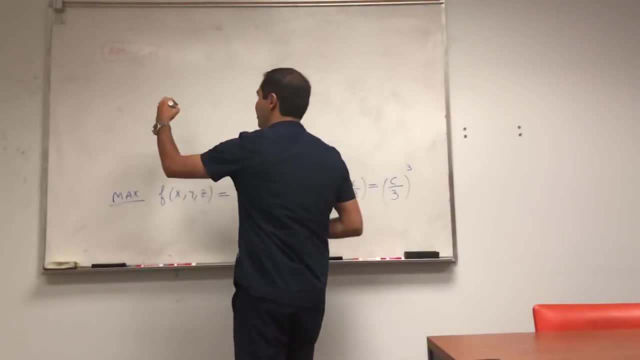 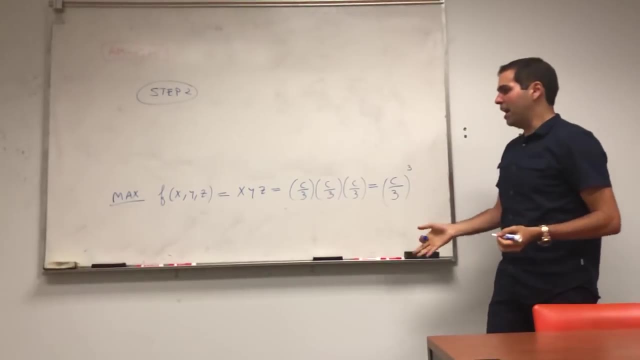 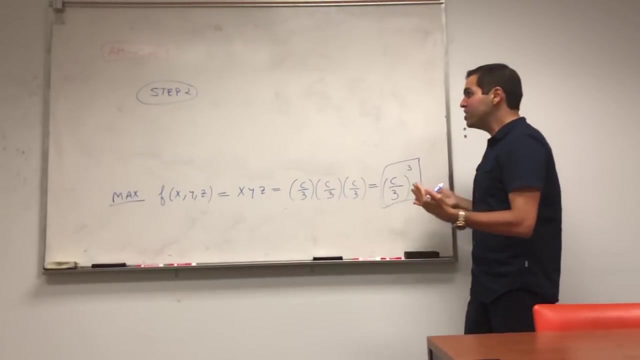 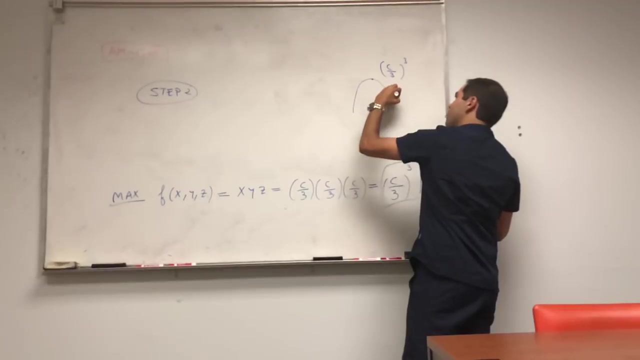 just extract some useful info from that. so step 2: okay, what do we have? we have again that this is the maximum value of F, but by definition of the maximum value again, suppose this is C over 3 cubed and this is, I guess, F of XYZ. 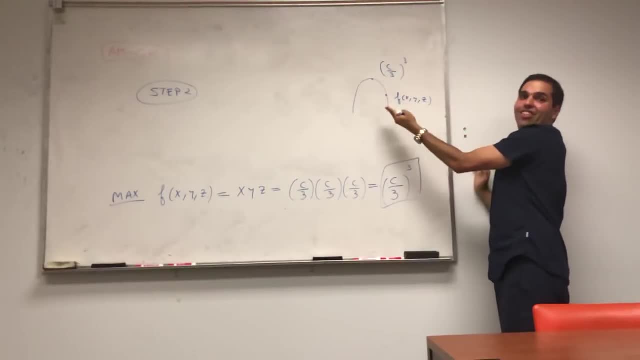 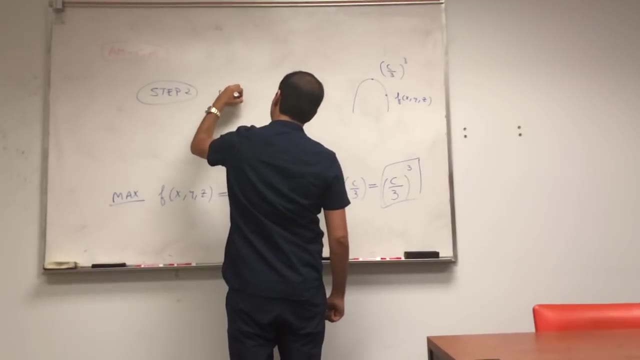 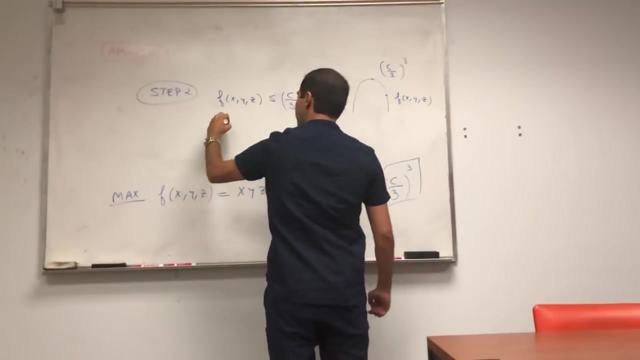 because this is the biggest value. any other value of F must be beneath it. so, by definition of a maximum, we have F of XYZ is less than or equal to C over 3 cubed, and so, in particular, XYZ is less than or equal to the cube root. sorry of. 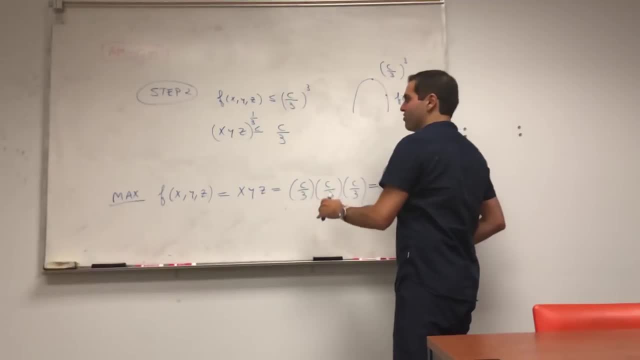 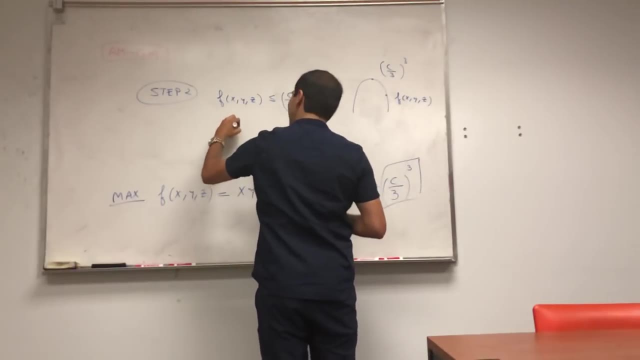 X plus or minus 1 X plus, So preventing the whole equation. so let's just write that out very cleverly: for what is equal to L over 3, cubed two into all the X where is less, or equal to c over 3.. Sorry again. So what we have is x, y, z is less, or 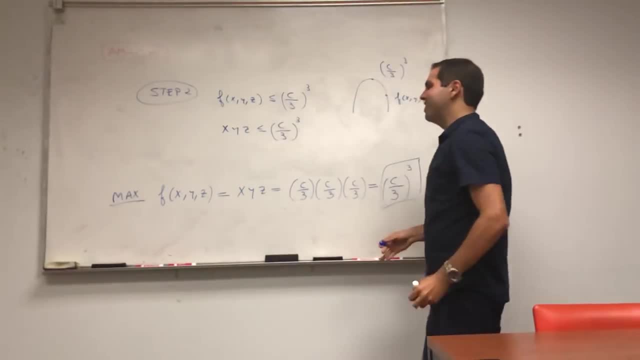 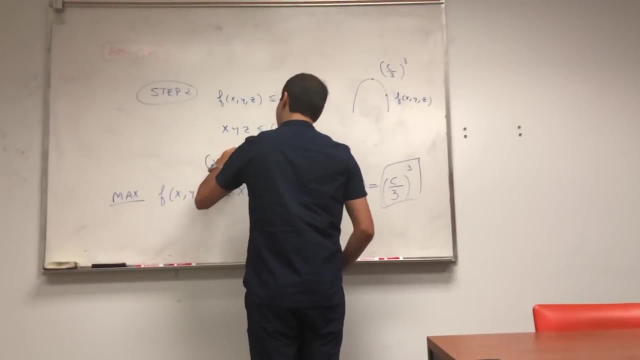 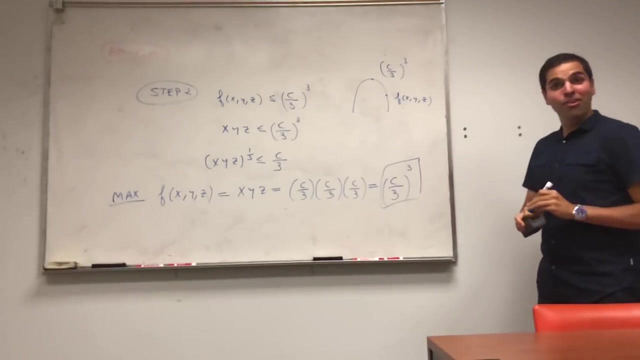 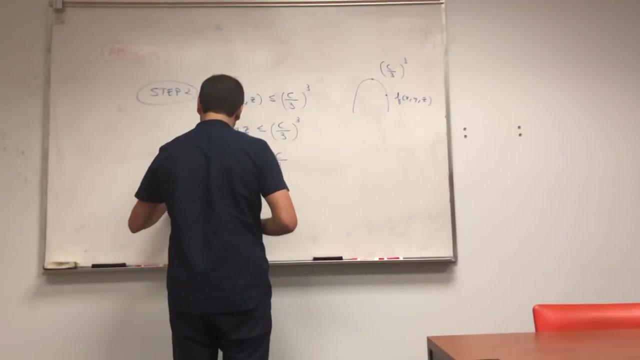 equal to c over 3 cube, That's by definition of f. Then take the cube root and you get the cube root of x, y. z is less or equal to c over 3.. And we're almost done, because what was c? Remember? c was just x plus y plus z, So we get x- y.